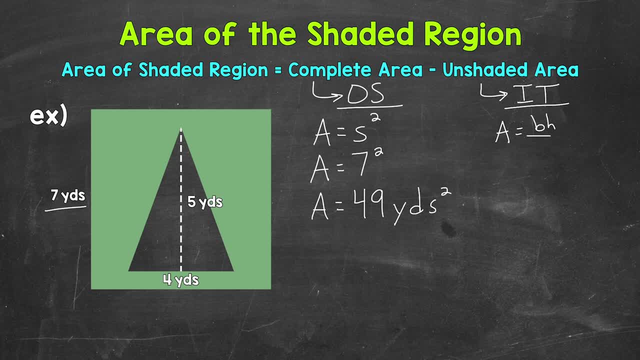 area equals base times height divided by 2.. Now for a triangle. you can also use one half times base times height. Both formulas will give you the correct area. Now let's plug in the base and the height. This triangle has a base of 4 yards and a height of. 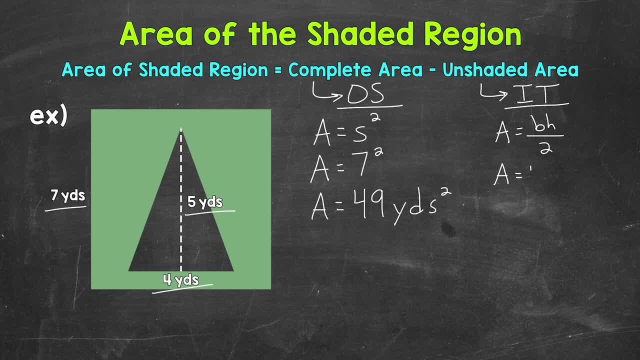 5 yards. So area equals 4 times 5 divided by 2.. Now let's work through this. We will start with 4 times 5, which is 20.. So we have 20 divided by 2.. That gives us an area of 10 square yards. Now we have. 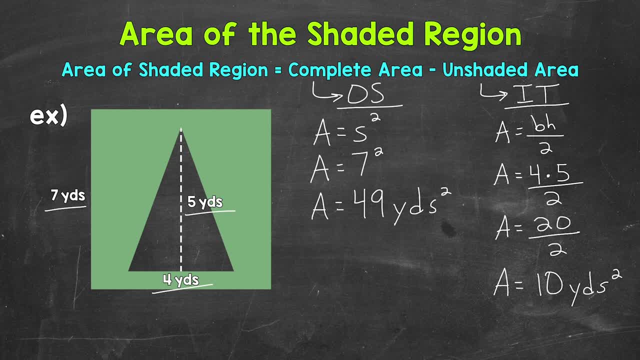 all of the information we need to find the area of the shaded region. We need to take the area of the outside square and subtract the area of the inside triangle, So 49 square yards minus 10 square yards. So for the area of the outside square we need to subtract the area of the inside triangle. 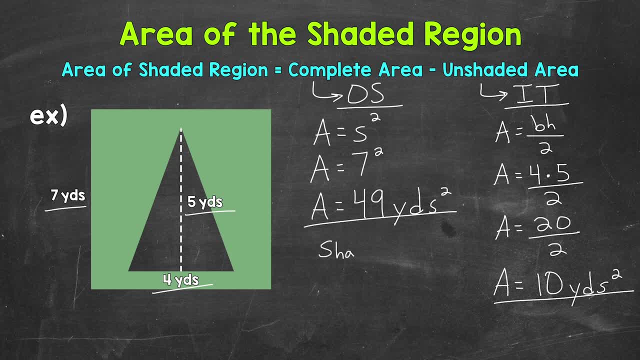 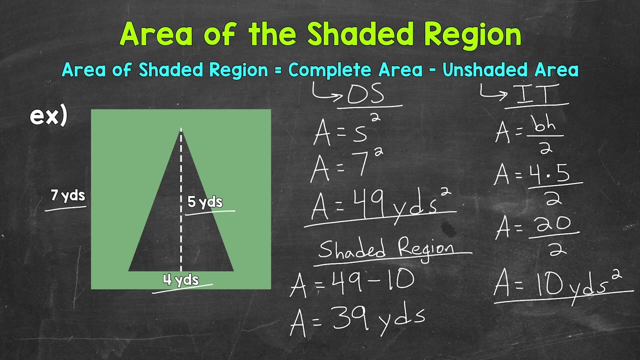 So for the area of the shaded region, I'll make a section down here. So this is going to be the area of the shaded region. We have area equals 49 square yards minus 10 square yards. 49 minus 10 gives us an area of 39 square yards. 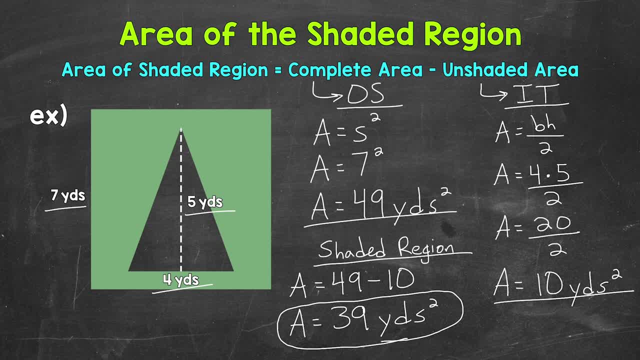 and this is the area of the shaded region. So, to recap, we found the complete area of the outside square, Then we found the area of the inside triangle and then, lastly, we took the area of the outside square and subtracted the area of the inside triangle. That gave us the area of 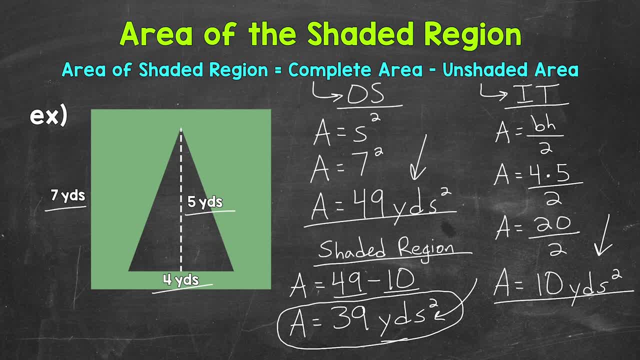 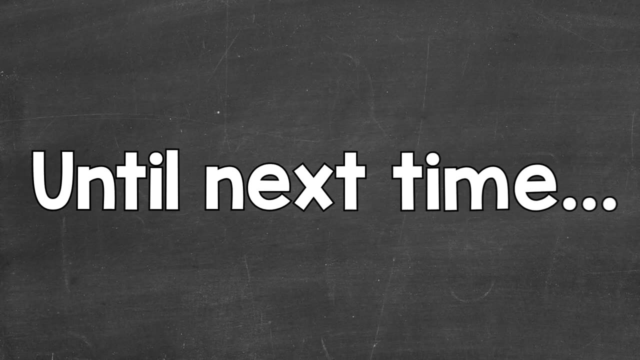 the shaded region. So there you have it. There's how to find the area of the shaded region. For our example, we took a look at a triangle inside of a square. I hope that helped. Thanks so much for watching. Until next time, peace.